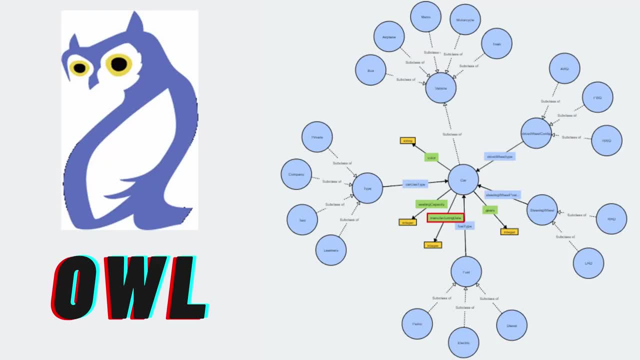 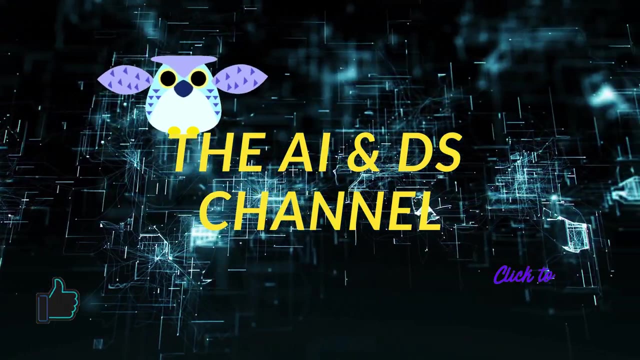 Hello and welcome back to another video. In this video we will have an introduction to OWL, an ontology language for schematic web, and then learn to visualize it using an online visualization tool. Stay tuned. You are watching the Artificial Intelligence and Data Science channel. Subscribe for more. 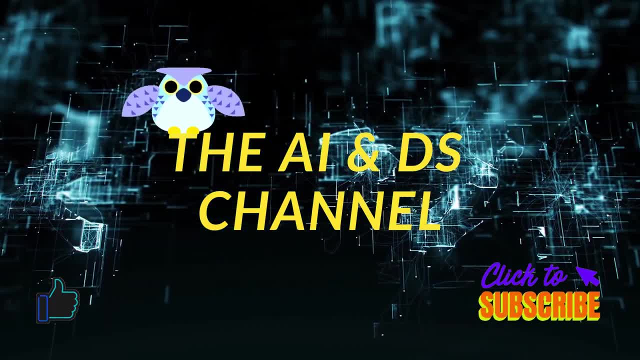 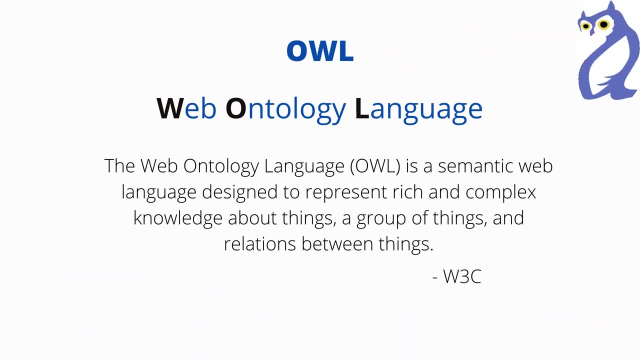 amazing videos. OWL stands for Web Ontology Language. Wait, isn't that W-O-L? Well, for easier abbreviation and pronunciation, W3C made it as OWL. The W3C formally describes OWL as a semantic web language designed to represent rich and 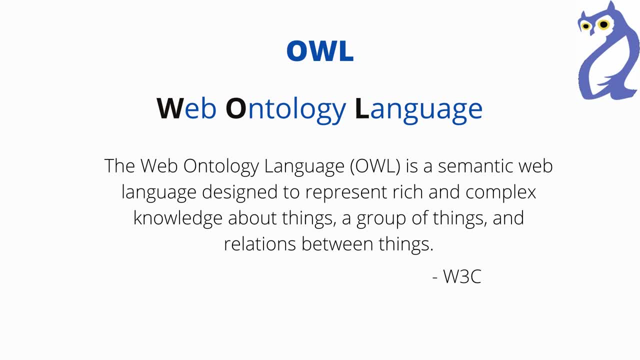 complex knowledge about things, group of things and relation between things. In simple words, we can say: OWL is a semantic web language which is designed to represent ontologies. It is one of the core semantic web standards, along with RDF and SPARC. here. 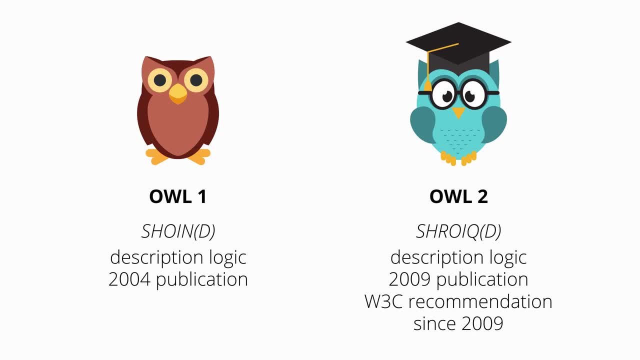 The current version of OWL, also referred to as OWL2, was developed by W3C Owl Working Group and was published in 2009, and this is the W3C recommendation since 2009.. OWL2 is based on a descriptional logic- SHROIKD- whereas OWL1 is based on a descriptional logic. 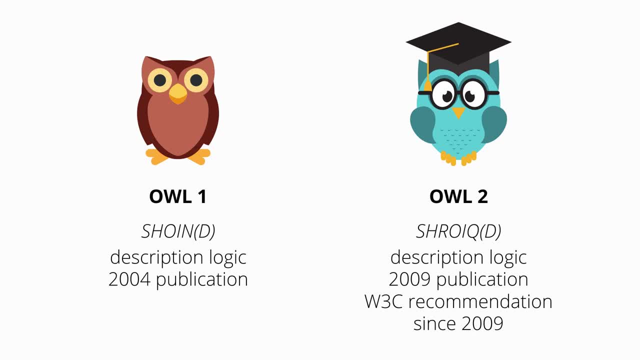 SHROIND. The OWL languages are characterized by formal semantics. They are built upon W3C's external standards for objects called RDF. OWL and RDF have significant applications in research, medical and commercial aspects. Speaking about ontologies, an ontology can be described as a way of showing the properties. 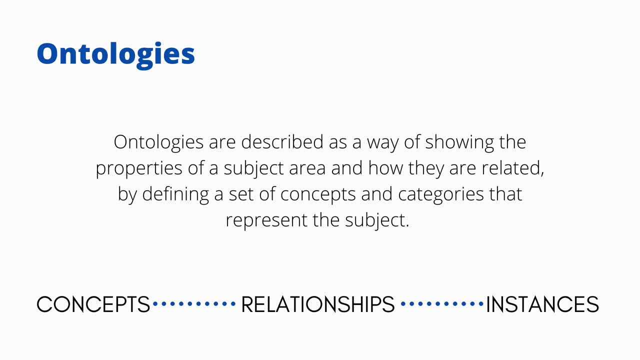 of a subject area and how they are related, by defining a set of concepts and categories that represent the subject. Every academic discipline creates an ontology to limit complexity and to organize the data in the form of a knowledge representation. New ontologies help to solve the problem within that domain. 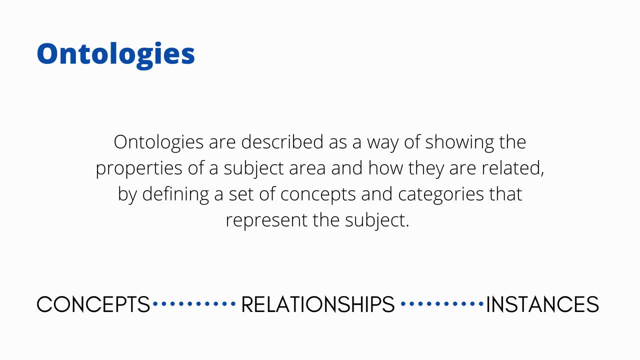 The main components of an ontology are concepts, relations and instances. It is similar to the triples format that we discussed in the semantic web video. If you want to know more about the semantic web technologies, check out my previous video on semantic web. 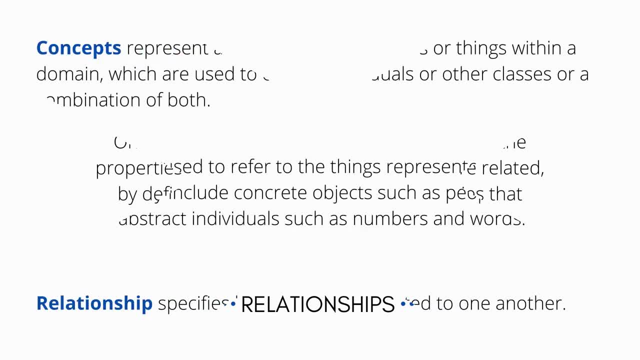 I will add a link to it in the description below. A concept represents a class or class of entities or things within a domain. Classes may classify individuals or others, classes or a combination of both. For example, Consider which is a class of all cars. 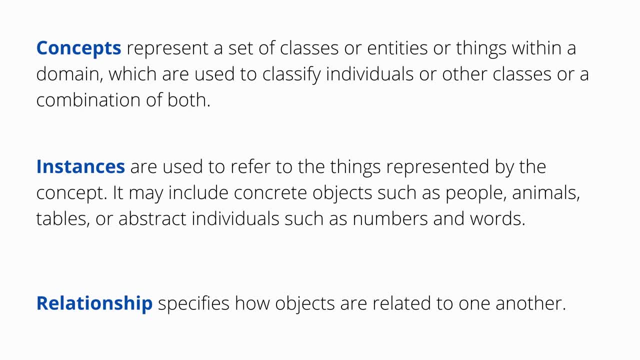 or an abstract object that can be described by the criteria of being a car. Another example is Thing, which is a class of all things, or an abstract object that can be described by the criteria of being a thing. explicit pursuit of advanced typical data 없어. 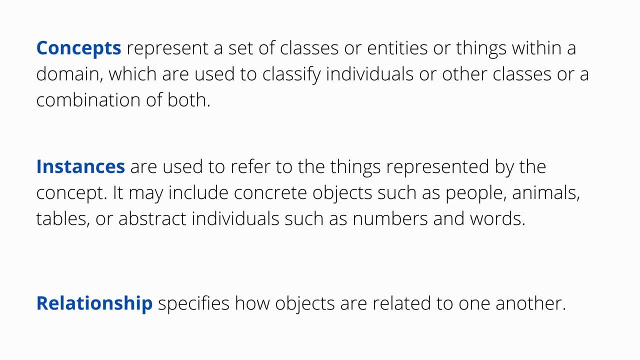 abstract individuals, such as numbers and words. Strictly speaking, ontologies need not include instances. as it is supposed to be a conceptualization of the domain, A combination of an ontology with an associated instance is known as knowledge base. Relationships in an ontology specify. 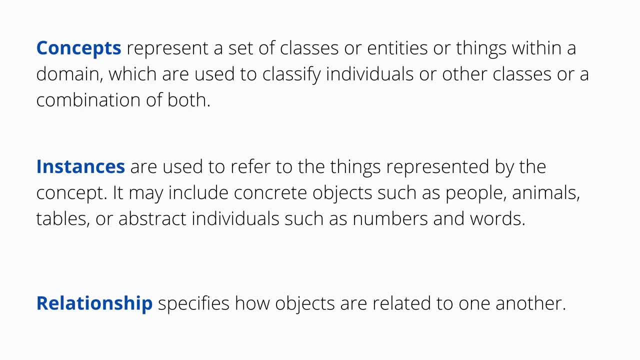 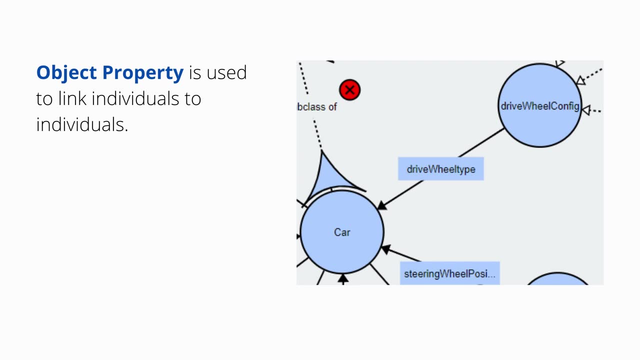 how objects are related to other objects. For example, John likes football. Here likes denotes the relationship between the object John and the object football. There are two types of properties that exist for our. They are object property and data type property. Object properties are used to link individuals to individuals As we 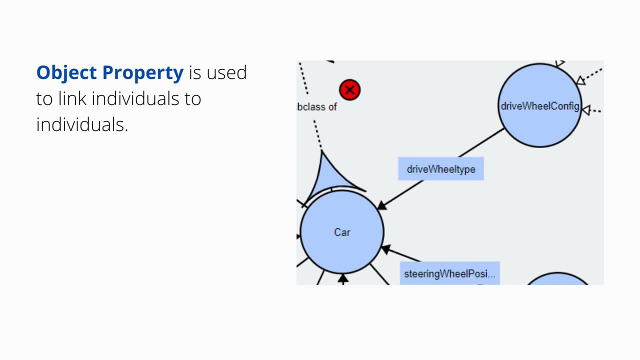 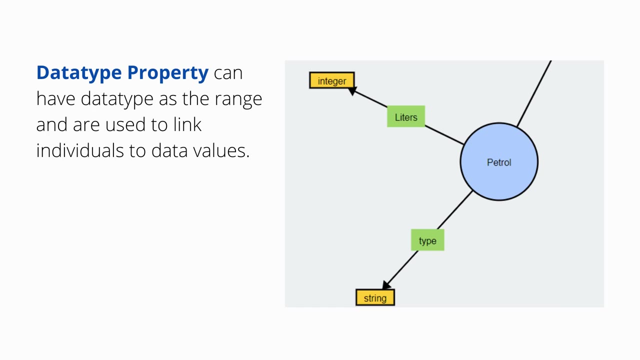 can see from the example, DriveVilleType is an object property that links DriveVilleConfiguration and Car. This indicates a different DriveVilleType available for the car. DataType property properties are used to link individuals to data values. data type properties can have data type as. 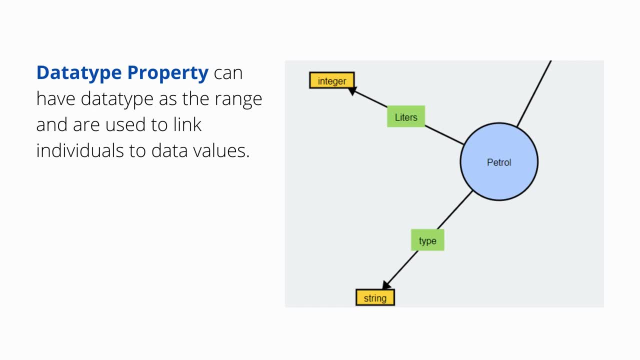 screens, as we can see here. letters is a data type property that can be used to denote the quantity of fuel that can be stored in a car, whereas type is a string type property used to denote the type of fuel used in the car, such as premium, extra premium or ordinary type of fuel. okay, since we 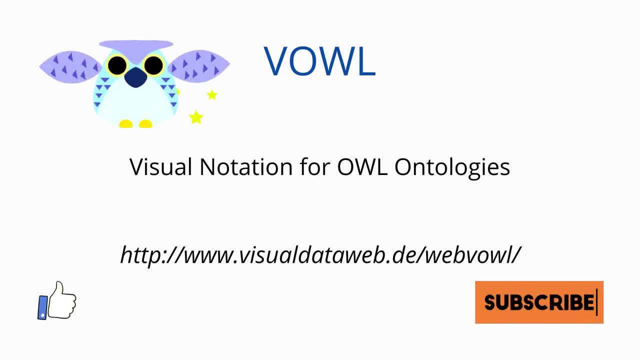 have a basic idea about out. let's try visualizing it in the online visualization tool, vr. i've added a link to vr online editor in the description below for you to check it out. let's start. so we are in the visualization page. we go to modes editing. 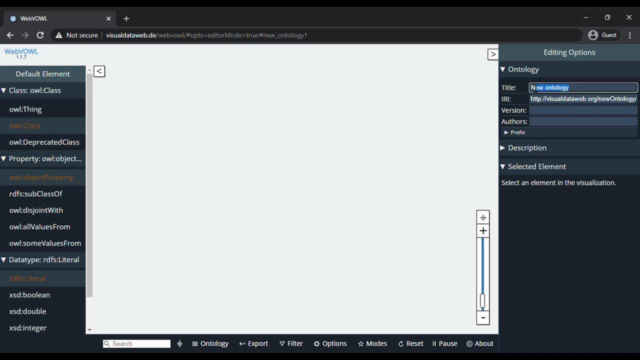 ontology. create new ontology. we'll create the ontology about vehicles. give a description. this is an ontology about vehicles. okay, then we go to class create: double click anywhere to create class. we create vehicle ontology to add subclass. you can go to subclass double click card and just drag and link it to get. 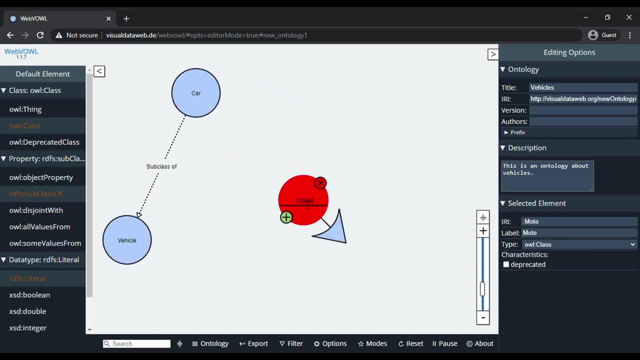 a subclass motorbike, airplane, bus, train. okay, now let's add object property for our class car, so that we go to object property and then we click here. we named as drive wheel configuration, configuration to indicate the different drive wheels. it adds subclasses for it or we'll drive. 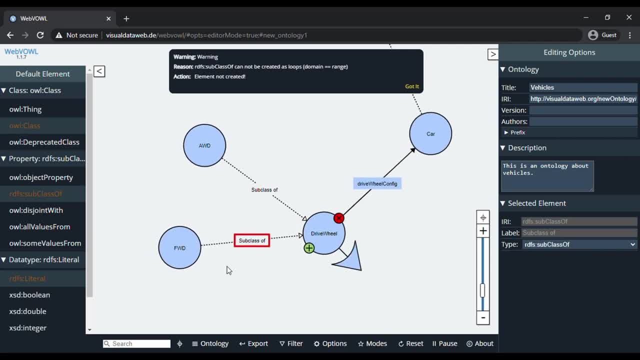 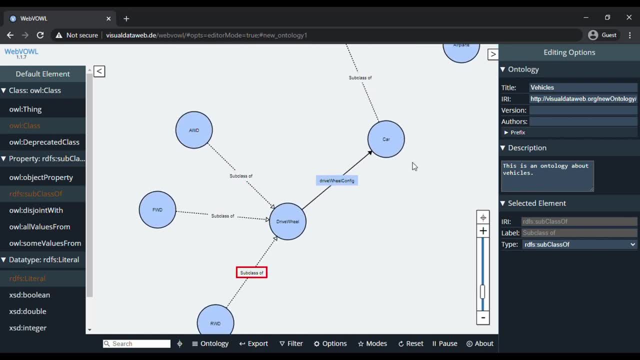 front wheel drive, rear wheel drive. we'll add another object type: object property sharing wheel. this is to show the steering wheel position and give subclasses: left hand drive, right hand drive. we'll add another subclass, object property fuel, to indicate the fuel type. fuel type: okay, and we'll add some classes. 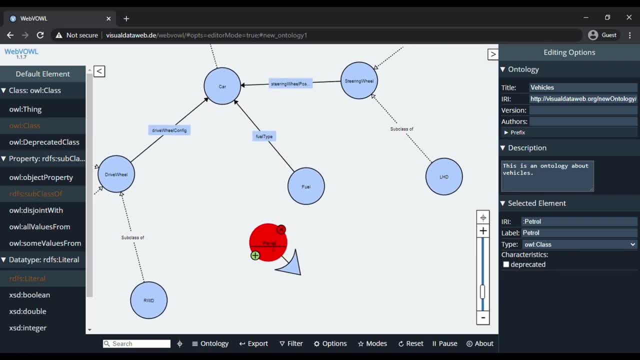 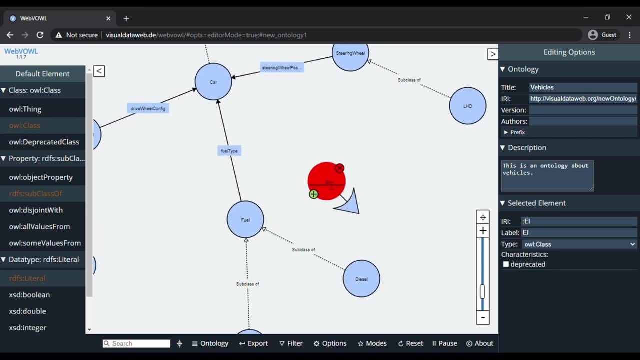 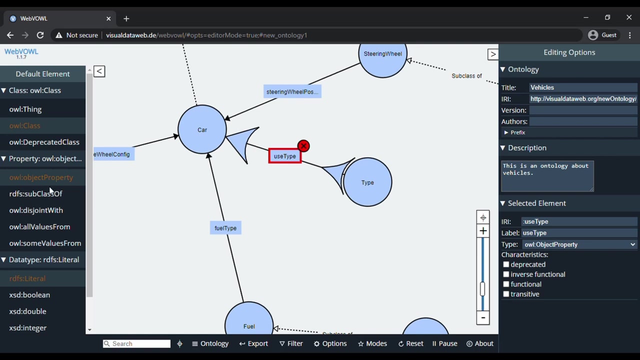 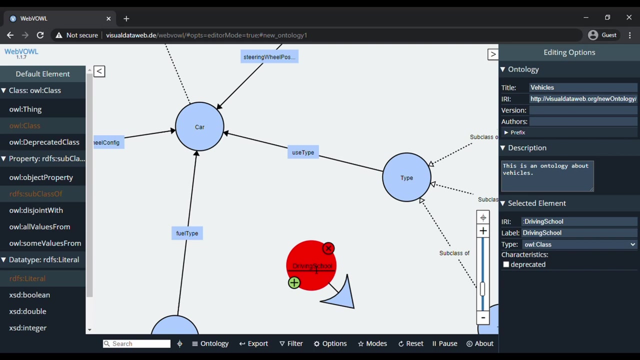 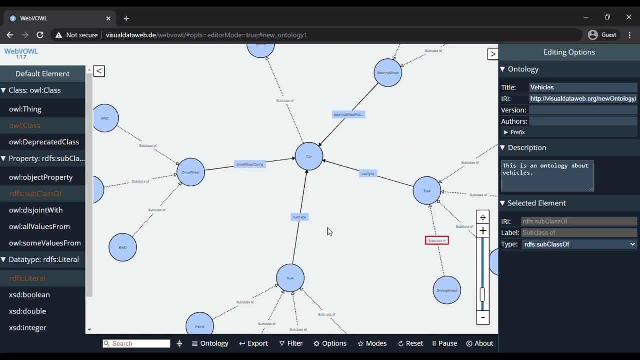 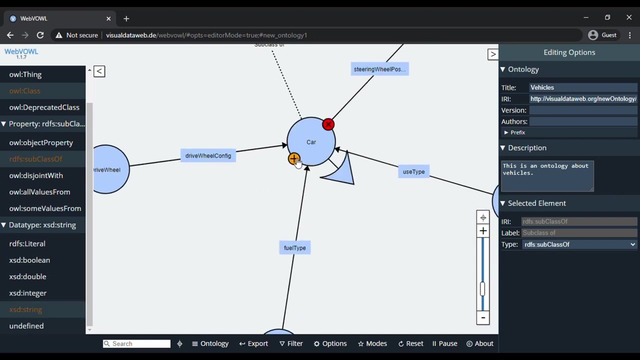 petrol, diesel, electric, hybrid. okay, now let's indicate the use type: object property type. indicate the use type: subclass: taxi, privately owned company, driving school. okay, now we have the basic object properties. let's define some data type properties today. let's start with the color. i go for a string, go here, click add data type property. 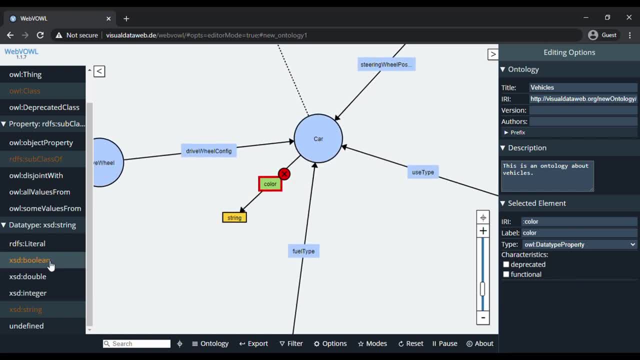 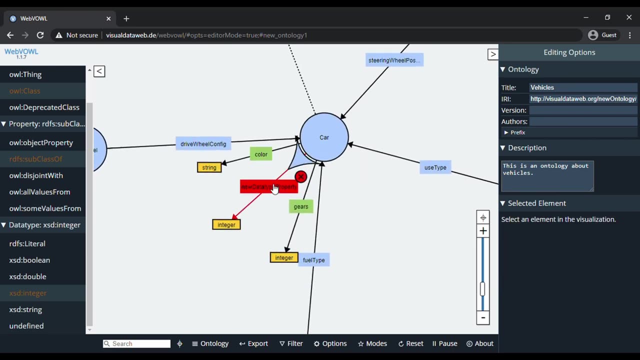 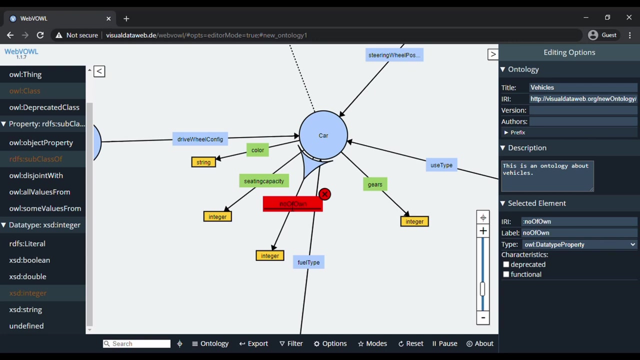 color. then let's give you the number of gears, which is an integer type, property gears. add one more: setting capacity. setting capacity: screw number of numbers. okay, there you have it, your basic visualization now. if you want to reduce gap, you can go to zoom control to change the gap between the objects. if you want to delete, 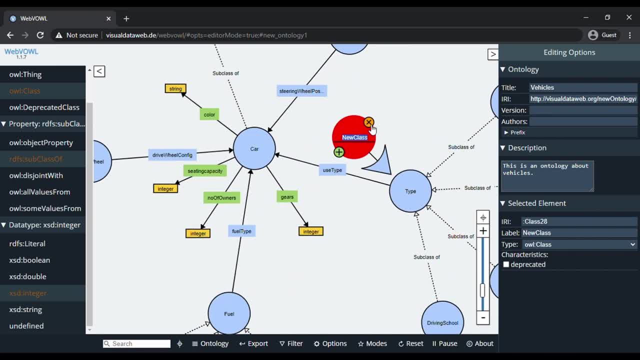 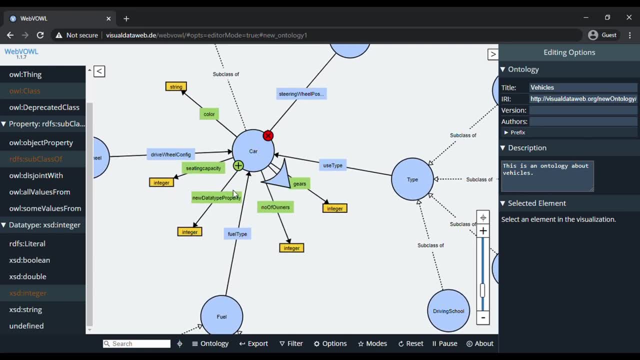 something, you can just click the x to delete it. hey, if i have an object property also, you can just delete it. so that is what you want to see. so for the object property you can just delete it. use some. sorry, if I have a data property, also, you can just delete it. there, you have a. 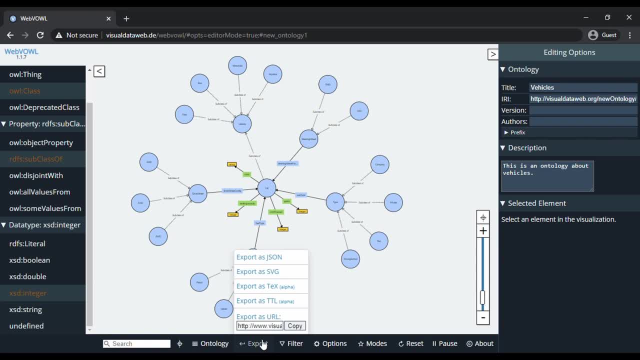 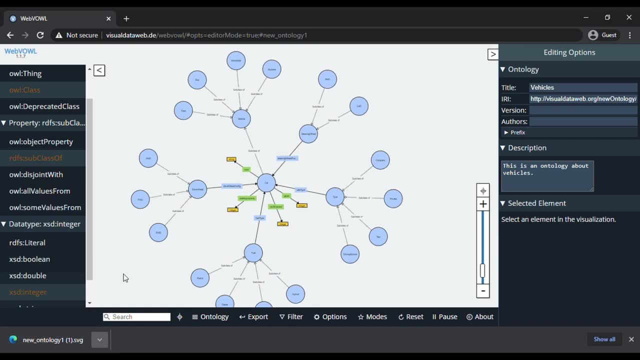 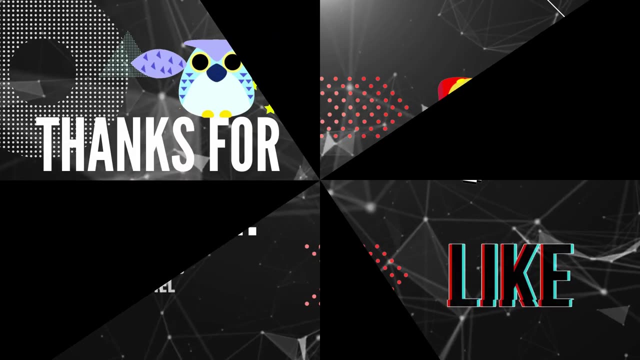 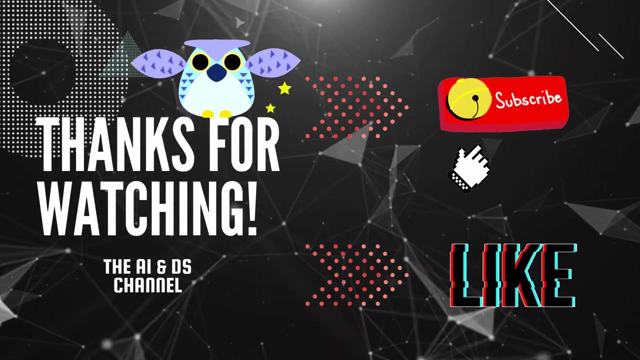 visualization now to export it. you can go to export and export it as any of the formats required. there you have it. that brings us to the end of this video. hope you got a basic idea about web ontology language and its visualization. see you in the next video.